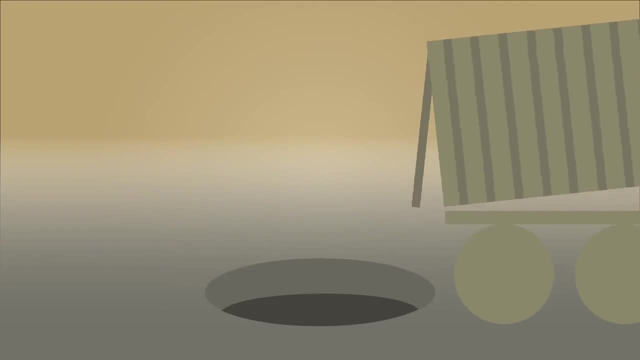 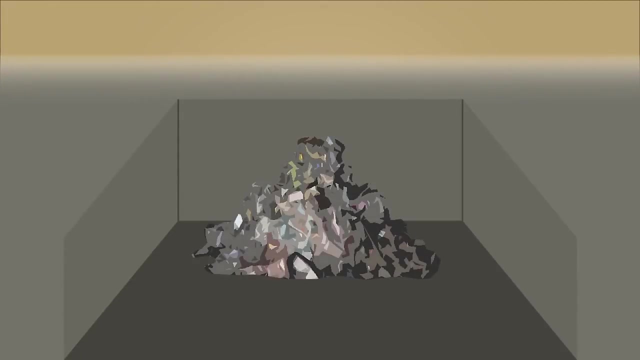 think that a landfill is an open hole in the ground where we bury the rubbish. you'd be wrong. In fact, it is a carefully designed structure built into or on top of the ground to store your rubbish in such a way that it will be isolated from groundwater, Our fresh 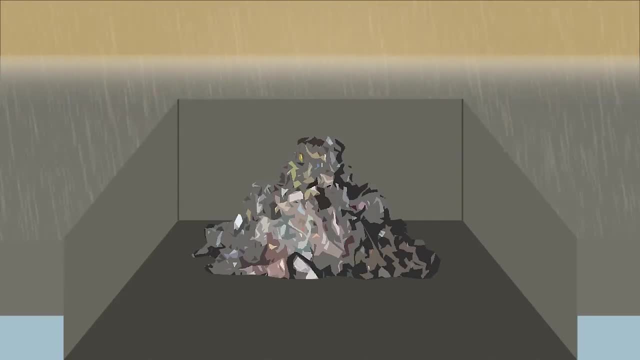 water supply will be kept dry, preventing leaking into this groundwater, and will not come into contact with the air, causing horrible smells. This isolation is achieved with a bottom liner typically made from very thick PVC, and a daily covering of soil. However. 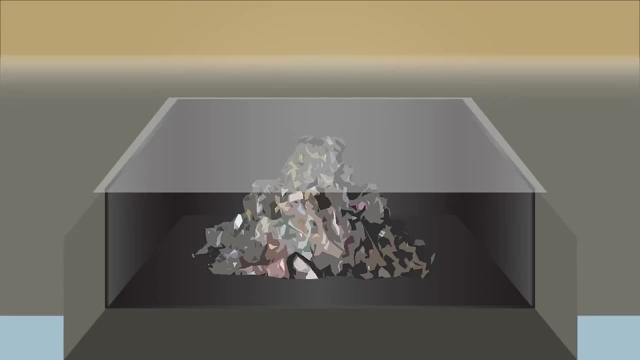 in many countries, open rubbish tips still exist, causing environmental and health problems. If our rubbish is isolated from the surrounding environment, it doesn't decompose. Landfill sites are not like a compost pile, where the purpose is to bury rubbish in such a way that. 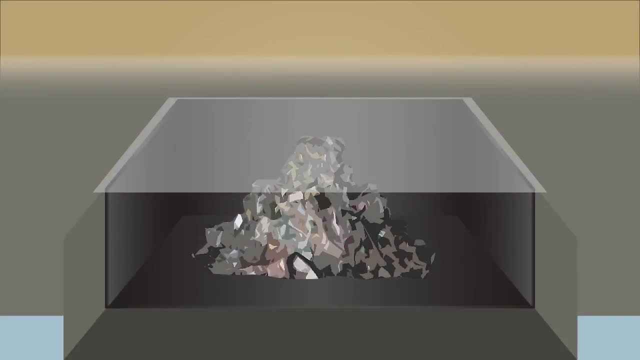 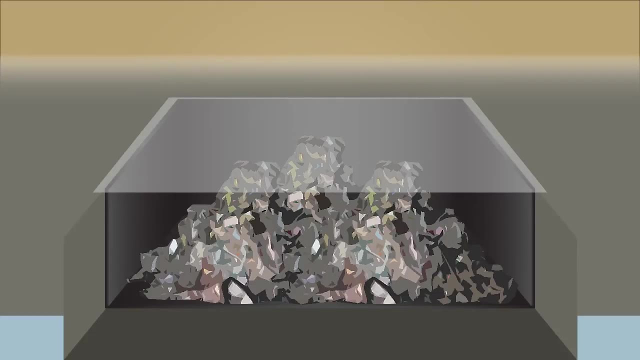 it will decompose quickly. Rather, landfill sites are simply a way that we cope with a vast amount of rubbish that we produce. Let's now take a look at the parts that make up a landfill cell and how these cells make up organised landfill sites. 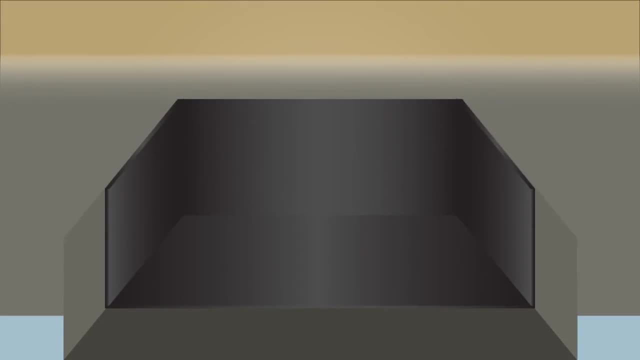 Groundwater has to be protected from chemicals found in our waste, and so compacted clay is placed on top to act as a physical barrier. On top of this is a very thick, waterproof plastic liner. This stops water that contains waste chemicals called leachate from contaminating. 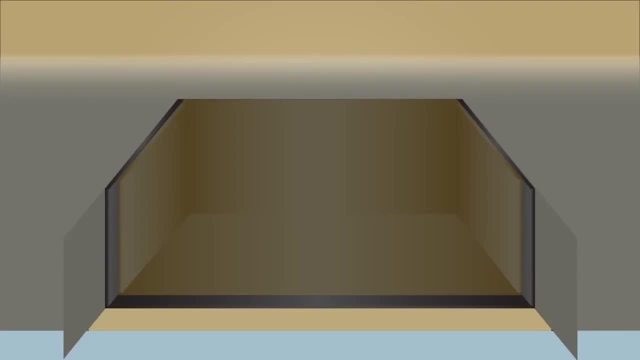 this groundwater, A geotextile mat, typically made from polypropylene or polyesters, are like a woven fabric, and this, too, prevents the plastic sheeting from being damaged by the sharp gravel layer as the rubbish on top is compacted. 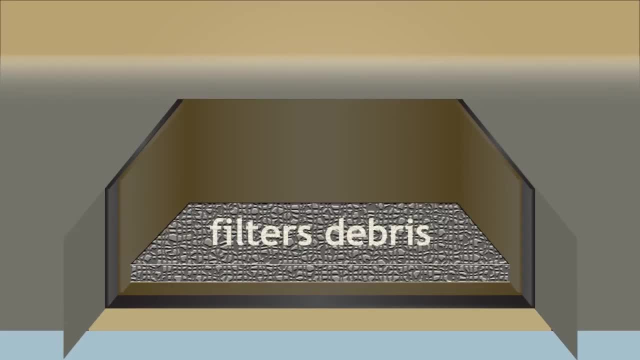 The gravel layer on top of the geotextile mat filters large pieces of debris, allowing only water through. This improves the drainage of the landfill cell. The gravel layer is connected to a leachate pipe. This is a very important part of a landfill cell because it is the only part of the landfill. 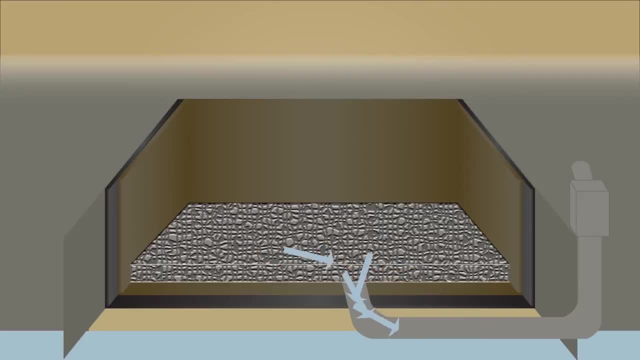 cell that has a leachate pipe. The leachate is collected through pipes, where it goes into a leachate pond. This leachate can't be used as drinking water and needs to be treated like sewage before it can be removed from the site. This must continue, even when